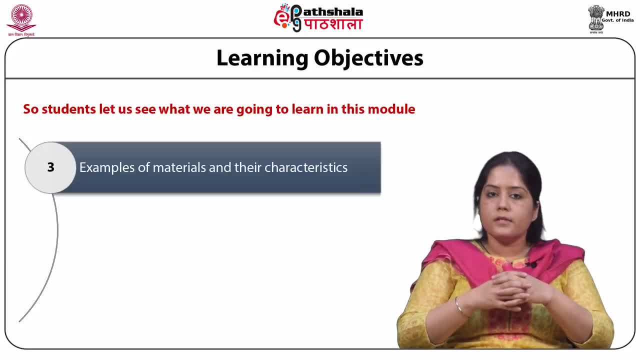 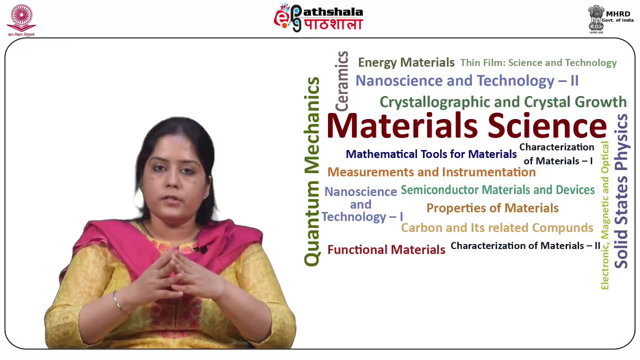 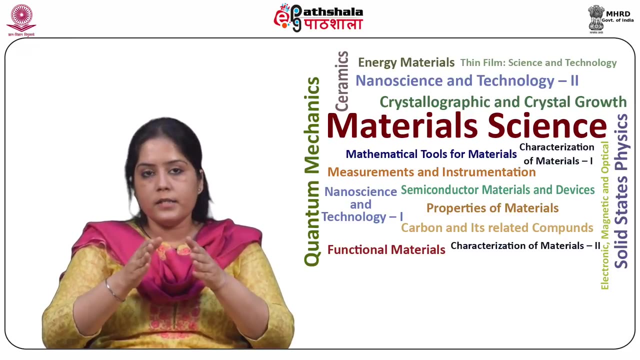 Lastly, we will also discuss about the application potential. So let us start with a brief introduction about this module. A feroid material is defined as a material which is exhibiting at least two of the ferroelectric or ferromagnetic or ferroelastic ordering in the single-phase state. 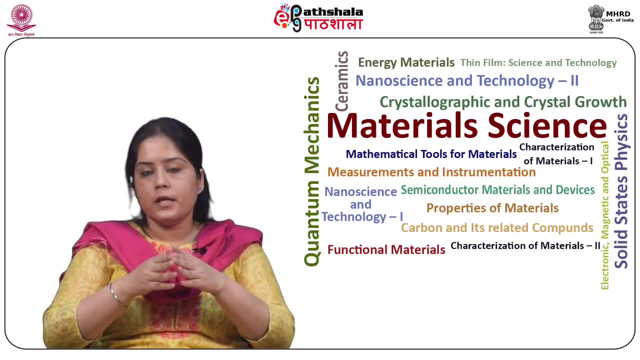 These ordering are typically manifested in the presence of a well-defined hysteresis. This means that the ferroelectric or ferromagnetic ordering is a single-phase state. This means that the ferroelectric or ferromagnetic ordering is a single-phase state. 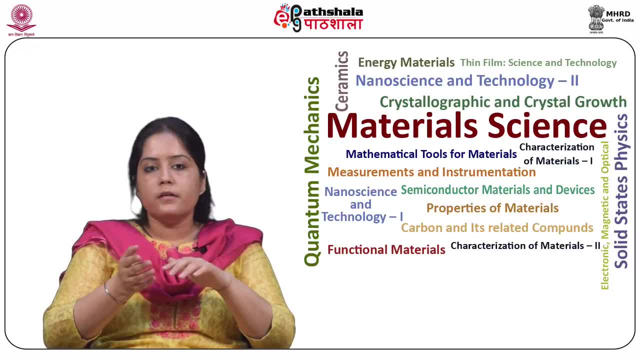 This means that the ferroelectric or ferromagnetic ordering is a single-phase state. This means that the ferroelectric ordering is a single-phase state When the material is switched under the bipolar electric field, magnetic field or mechanical stress. More recently, ferroelectric ordering, another ordering mechanism, has been proposed. 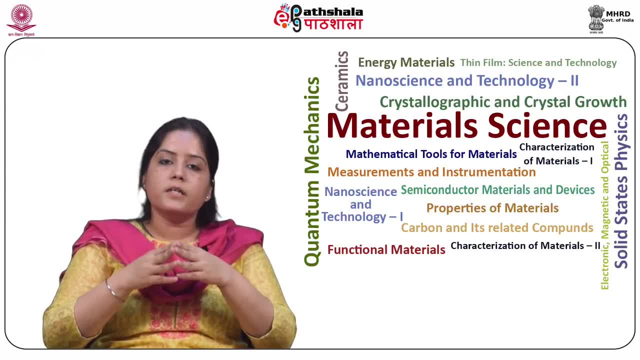 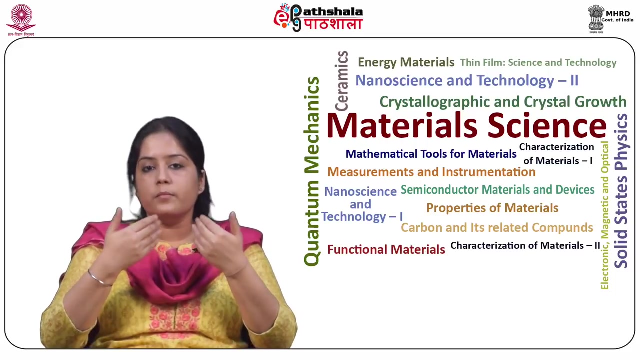 On the other hand, magneto-electric coupling in the materials is a general phenomena which could be present whether or not the material exhibits the magnetic or electrical ordering. For example, it could occur in the para-electric ferromagnetic materials, or it can be mediated by other parameters such as strain. 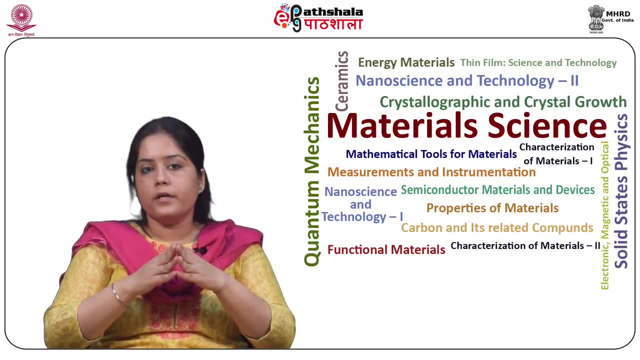 Hence the term. multi-feroic would mean a material exhibiting two or more of the above ordering mechanisms. More recently, multi-feroic materials have raised tremendous research interests because of their potential for several exciting device applications. Examples include the multi-state memory element or sensors or spintronic devices. 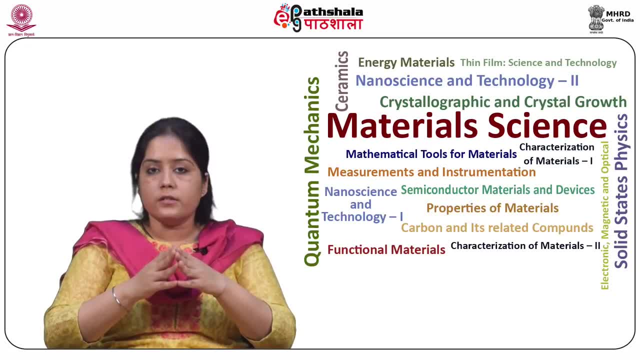 However, there are several challenges, As there are not many naturally occurring materials which shows multi-feroism, and hence most are artificially prepared in the laboratories. In addition, most of the materials shows transition temperature, which are below the room temperature, making these devices difficult to use. 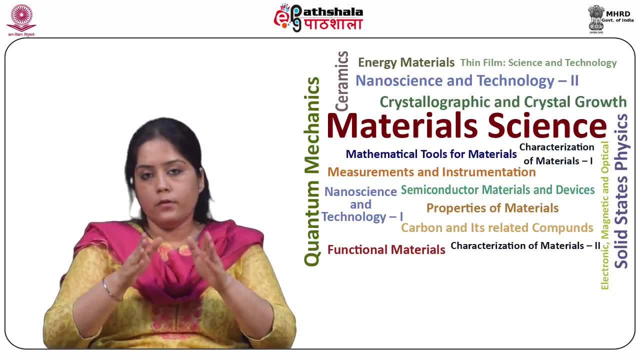 It also makes operation impractical. Also, there could be issues with respect to their fabricability in pure phase form. However, despite these challenges, researchers' quest remains to develop such materials, simply because they offer a practical and user-friendly solution. However, despite these challenges, researchers' quest remains to develop such materials, simply because they offer a practical and user-friendly solution. 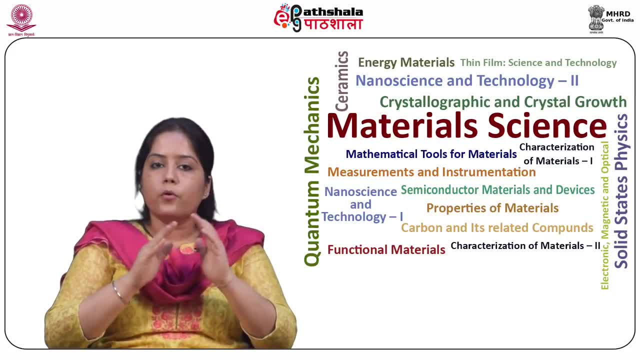 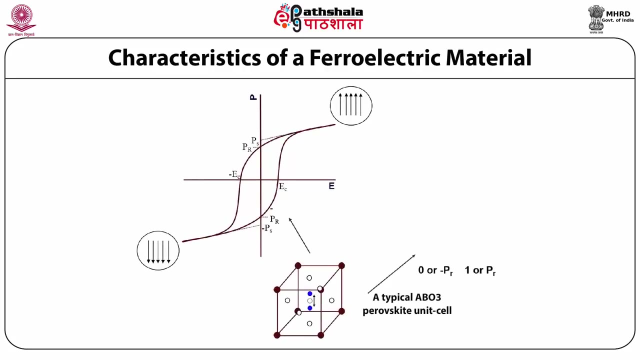 exciting opportunities from both the fundamental and application perspectives. So we are going to study some of the basic aspects of multi-ferroic materials and the attributes of a few example materials. Let us start with the characteristics of a ferroelectric material. The figure shows the ideal PE hysteresis loop for a ferroelectric material. 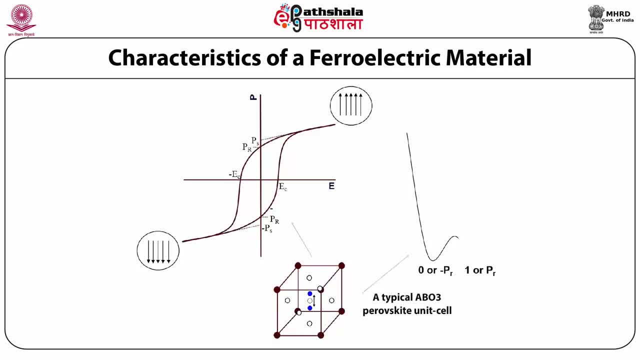 where the saturation polarization, that is, plus PS, corresponds to the state when all the spins are aligned parallel to each other and minus PS corresponds to the anti-parallel spins. The structure shows a typical ABO3 perovskite unit cell, which is a well-known ferroelectric material. 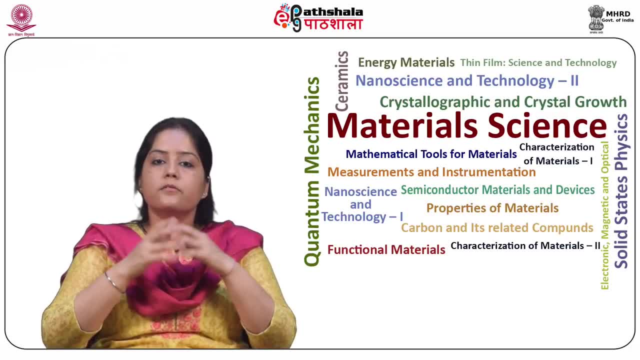 So now we will study about the ferroelectrics. Let us discuss about the four properties of ferroelectric materials and then we will study their applications. First, they are non-ferroelectric, They are non-centrosymmetric. Second, reversal of polarization and deformation by varying the 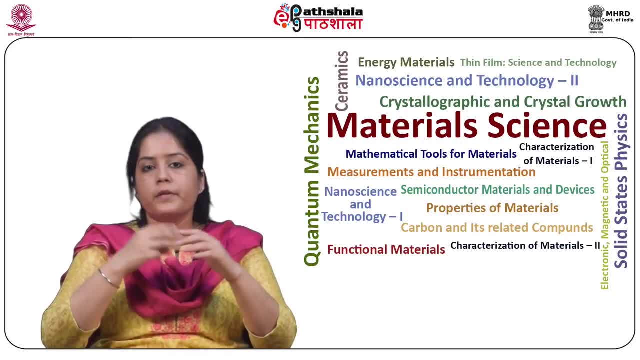 electric field and stress. Third, they exhibit the spontaneous polarization in the absence of electric field. Fourth, they also follows the Curie-Weiss behavior. Now they are applications. They can be used as sensors, actuators and transducers, Capacitors. 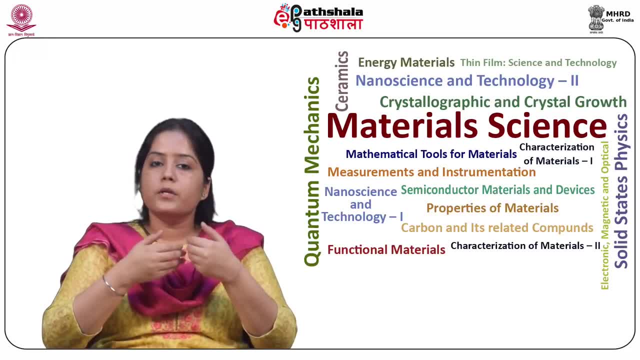 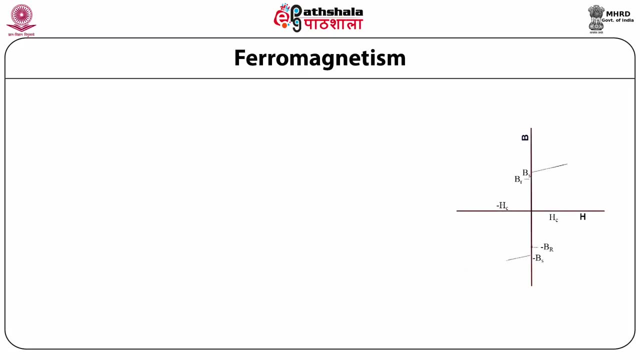 because they have high K dielectrics. They can be used in memories, for example non-volatile memories In the case of field effect transistors, or they can be used in microwave applications. Ferromagnetism, The spontaneous magnetization in the absence of magnetic field, is referred as the ferromagnetism. 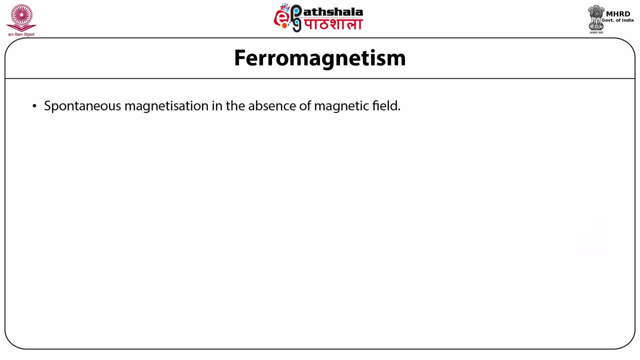 Now, as we can see from this B versus H curve, which shows that the saturation B, that is, the saturation magnetization BS, corresponds to the alignment of magnetic spins parallel to each other, Whereas minus BS, which are in the opposite direction, The ferromagnetism is used in transformer cores, permanent magnets, electromagnets. 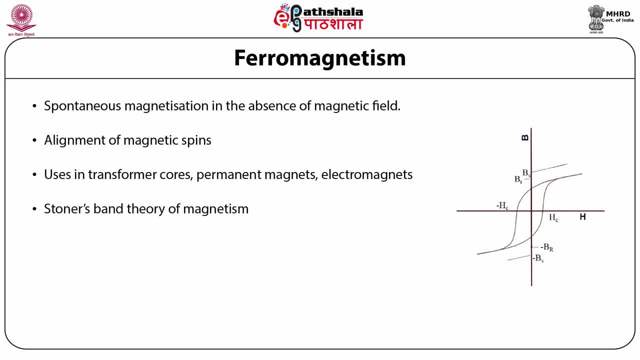 The Stoner's band theory explains the ferromagnetism, which describes there are three types of exchange interactions. The first one is called the ferromagnetism, The second one is called the intermagnetism, The third one is called the intermagnetism, The fourth one is called the. 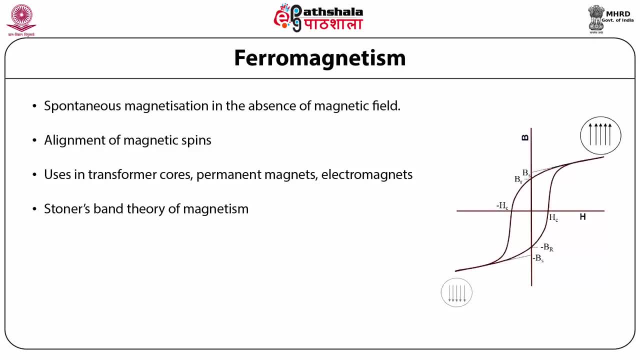 intermagnetism. The fourth one is called the intermagnetism. The fifth one is called the exchange interaction. First is the exchange interaction. Second, exchange energy, which is basically the driving force. Third is the exchange effect which dominates over the band. 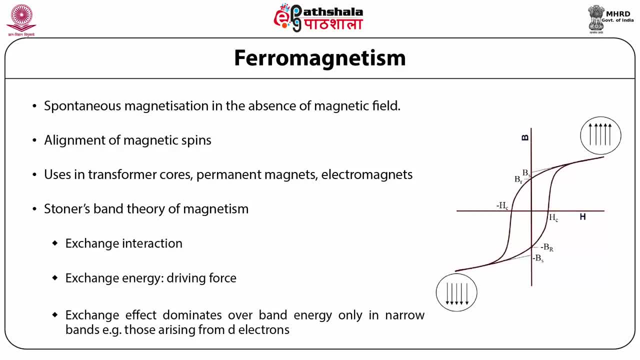 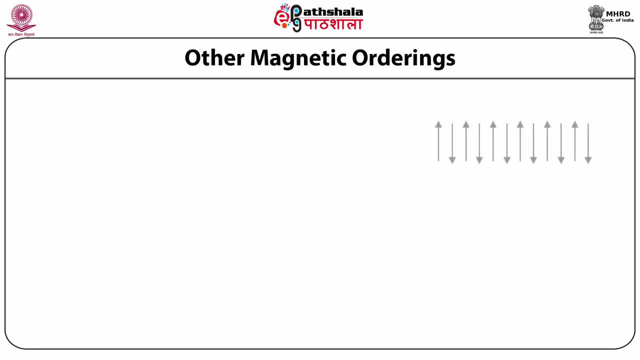 energy only in the narrow bands. Example: those arising from D electrons. Other magnetic orderings: Other magnetic orderings. Now, students, let us discuss about the other magnetic orderings leading to anti-ferromagnetism and ferromagnetism effects. First, we will discuss about the anti-ferromagnetism Here. 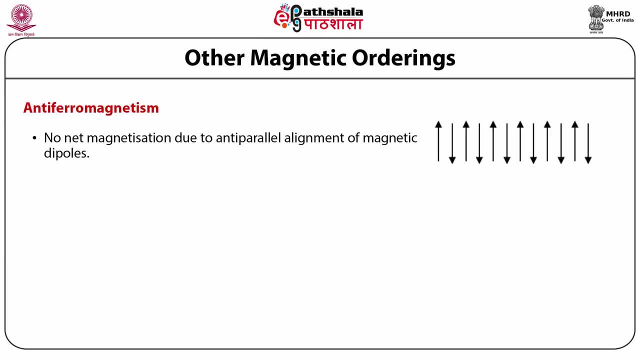 there is no net magnetization due to anti-parallel alignment of magnetic dipoles, which is shown in the physical diagram in the figure also, The examples of anti-ferromagnetic materials are chromium, manganese, manganese oxide, manganese sulfide and iron oxide. Next is ferrimagnetism, where 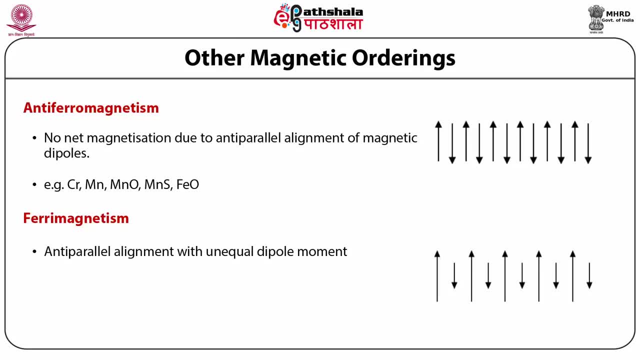 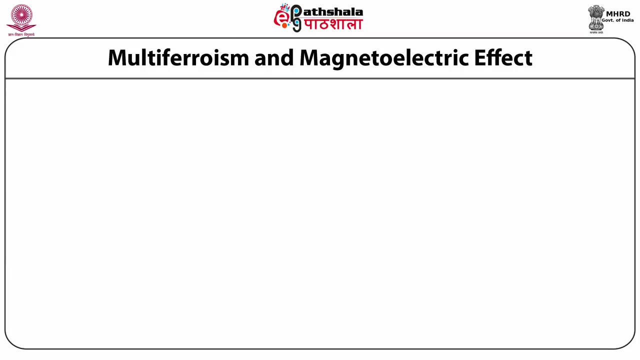 there is the anti-parallel alignment with unequal dipole moment. This leads to some remnant magnetization. The example of ferrimagnetism are ferrites. Now let us discuss about the two major effects, that is, multiferoism and magneto-electric effect. 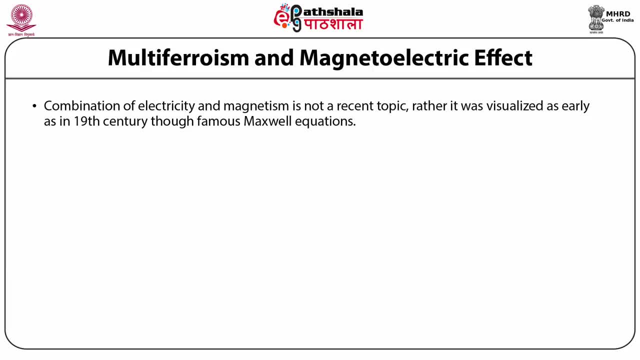 The combination of electricity and magnetism is not a recent topic. rather, it was visualized as early as in 19th century through famous Maxwell's equations. However, in most cases, electrical and magnetic ordering in solids are considered to be independent of each other. 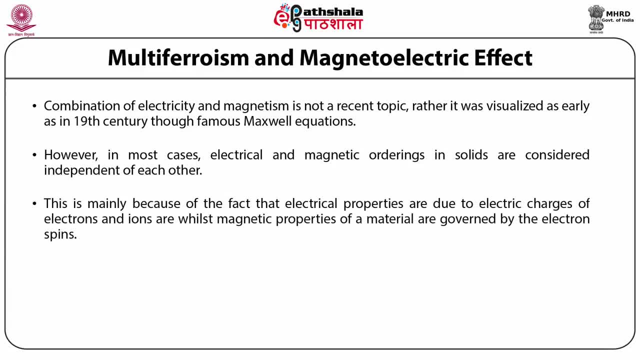 This is mainly due to the fact that the two types of energy of electricity and magneto-electric- mainly because of the fact that electrical properties are due to electric charges of electrons and ions are, whilst magnetic properties of a material are governed by the electron spins, Recent years have seen cases where the two 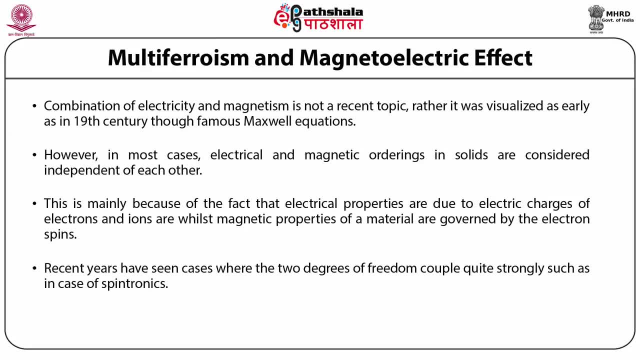 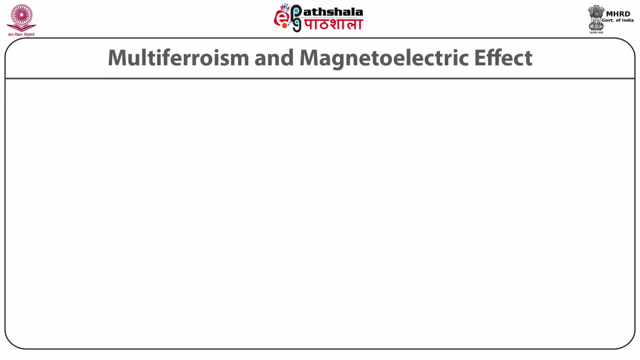 degrees of freedom couple quite strongly, as in the case of spintronics. In spintronics one can make devices where transport current can be manipulated by controlling the spins of electrons and vice versa. As Comiskey notes that although evidence of a strong coupling between electrical and magnetic degrees of freedom in insulating 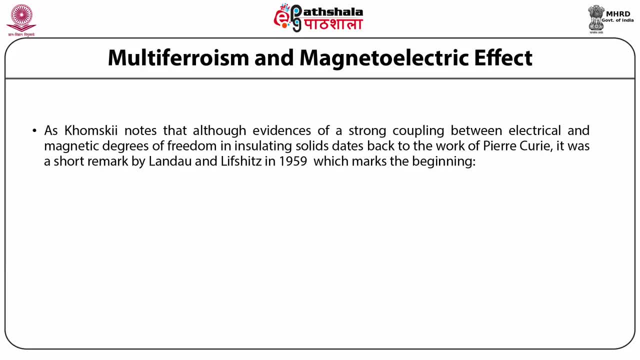 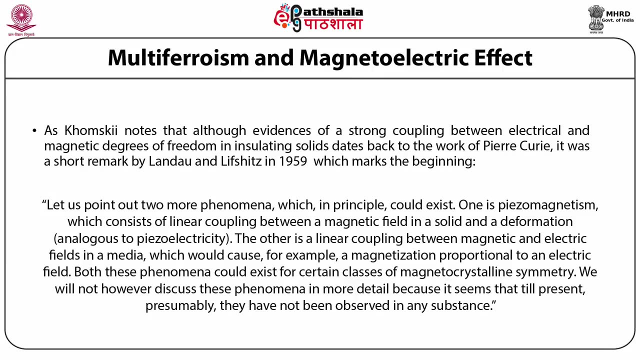 solids dates back to the work of Puri Curie. It was a short remark by Lando and Lifshitz in 1959 which marks the beginning. Let us point out two more phenomena which in principle could exist. 1. Piso-magnetism consists of linear coupling between a magnetic field in a solid and a. 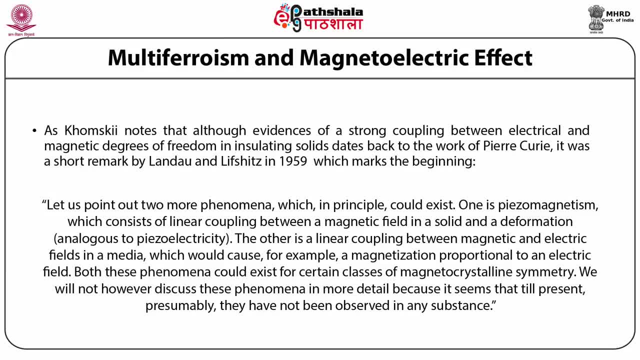 deformation analogous to piezoelectricity. 2. Linear coupling between magnetic and electric fields in a media which would cause, for example, a magnetization proportional to the magnetic field. 3. Linear coupling between a magnetic field and an electric field. 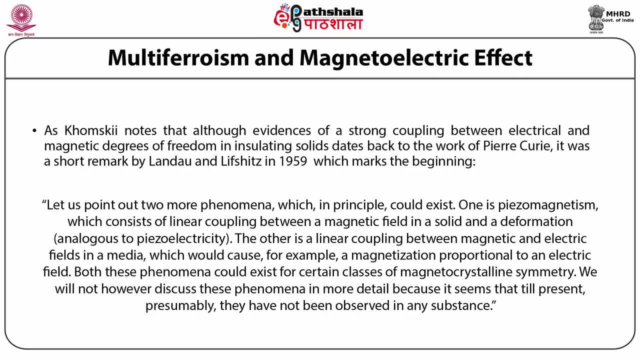 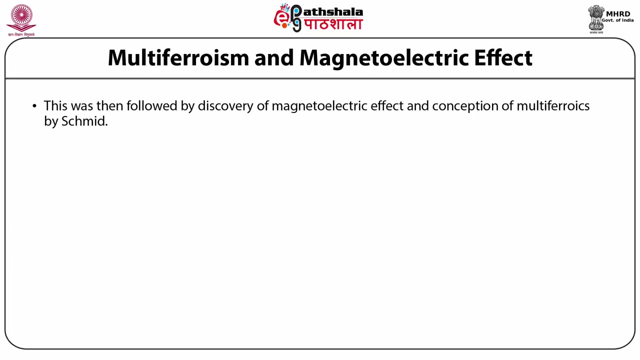 Both these phenomena could exist for certain classes of magneto-crystalline symmetry. We will not, however, discuss these phenomena in more detail, because it seems that till present, presumably they have not been observed in any substance. This was then followed by the discovery of magneto-electric effect and the concept of multipheroics. 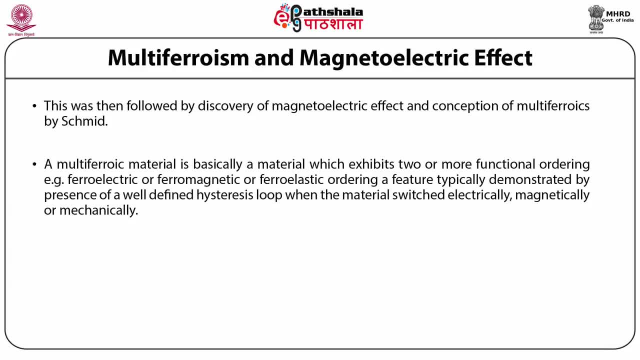 So a multipheroic material is basically a material which exhibits two or more functional ordering, eg. ferroelectric or ferromagnetic or ferroelastic ordering, a feature typically demonstrated by the discovery of magneto-electric effects and the concept of multipheroics. 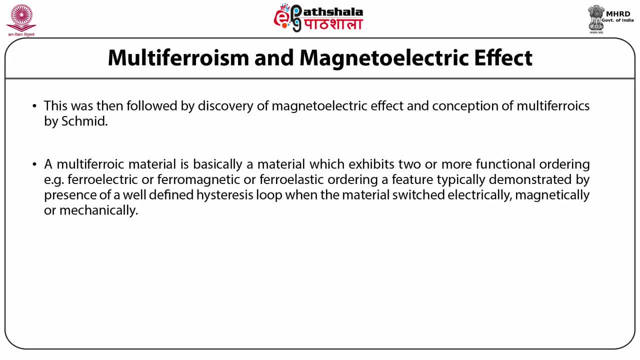 by the presence of a well-defined hysteresis loop when the material switched electrically, magnetically or mechanically. Next is the magneto-electric effect. Magneto-electric coupling in the materials, on the other hand, is a more general phenomenon, irrespective of the state of magnetic and electrical ordering, For example, 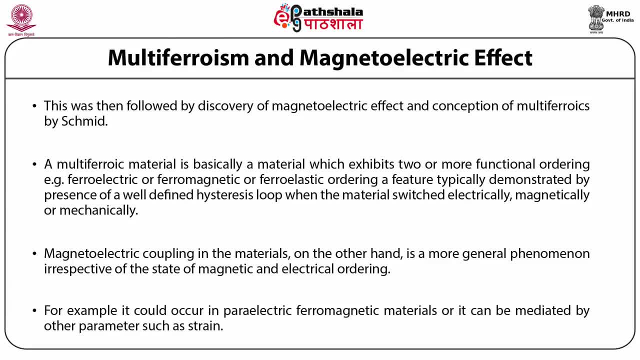 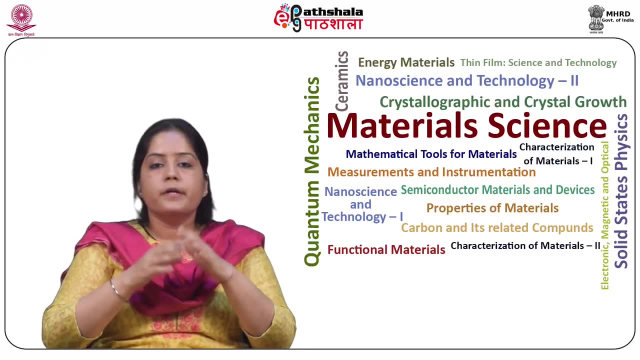 it could occur in para-electric ferromagnetic materials or it can be mediated by other parameters such as strain Multiferoics. The simultaneous existence of ferromagnetic ferromagnetic material in the plastic field gives the electric field asized potential to. 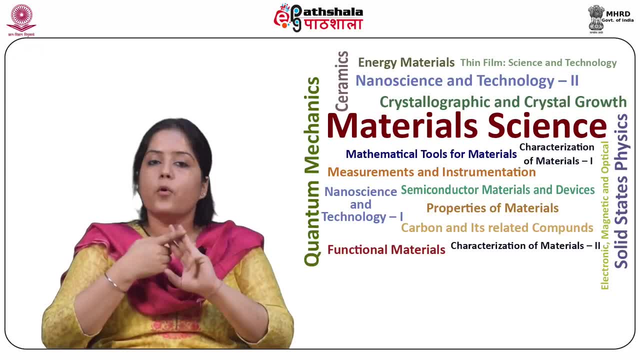 gradually increase the magnetic field. In physics, such auffled metal Stellebius would produce one and two-sidedезде möglich degrees of coordinates In quantum mechanics. they contribute unfaithfulness and they contribute vertical details and causes other forces to electric」. 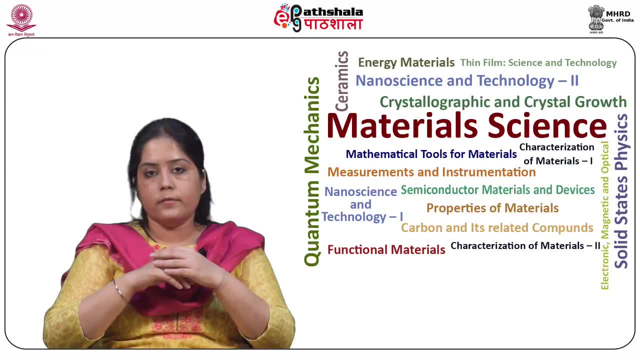 Thanks for watching. in device fabrication There are very few materials which exhibit this effect in a single phase form. Now they have variety of applications. First, sensors and actuators with additional degree of freedom in operation. Second, multi-state memory devices. Third, electrically controlled magnetic resonance devices. 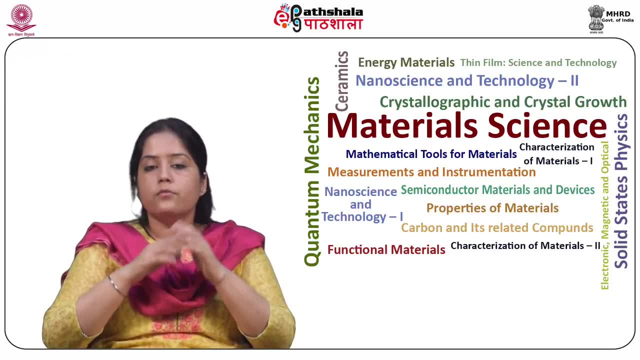 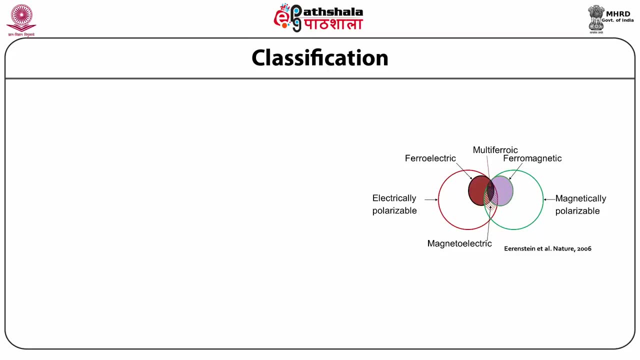 Fourth: transducers with magnetically modulated piezoelectricity. Fifth: spintronic devices. The classification of multi-ferroic materials and magneto-electrical materials. The figure explains the various possible scenarios. While there are a large number of magnetically and electrically polarizable materials, 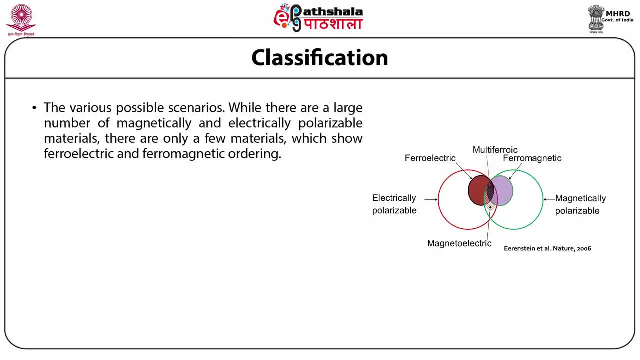 there are only a few materials which show ferroelectric and ferromagnetic ordering. Magneto-electric materials are those materials that are simultaneously electrically and magnetically polarizable, While multi-ferroic materials are strictly those type of materials which exhibit simultaneous presence of ferroelectric. 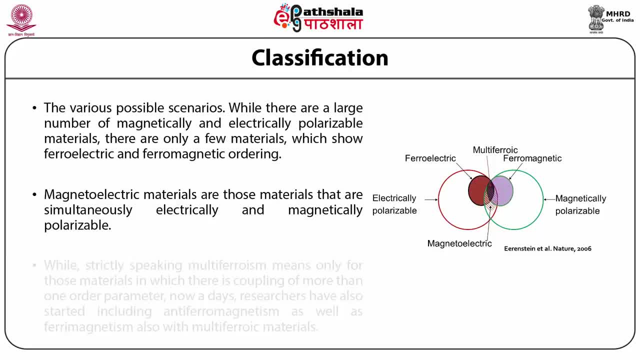 and ferromagnetic ordering, While strictly speaking, multi-ferroism means only ferroelectric ordering For those materials in which there is coupling of more than one order parameter. Nowadays, researchers have also started including anti-ferromagnetism as well as ferrimagnetism. 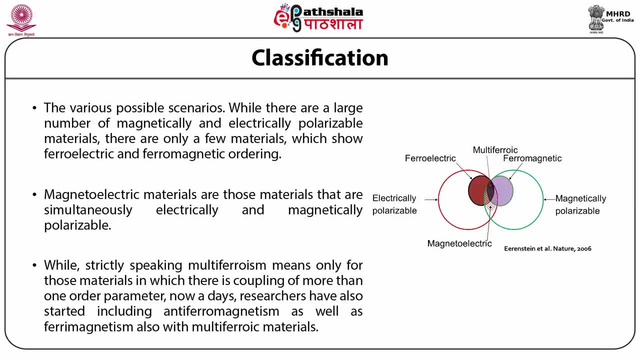 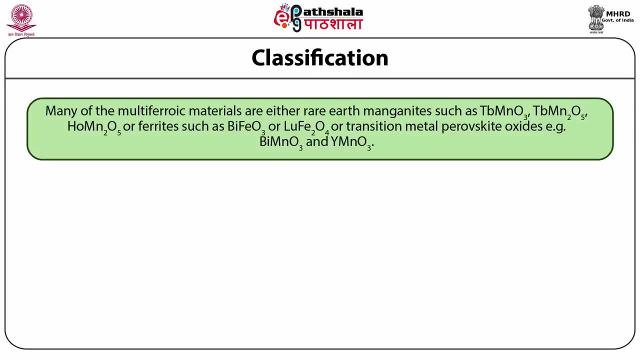 also with multi-ferroic materials. Many of the multi-ferroic materials are either rare-earth or metallic. Some are also non-ferroic. There are manyガ. These are the mainerei. take a look at different types of magneto-electrolysis. 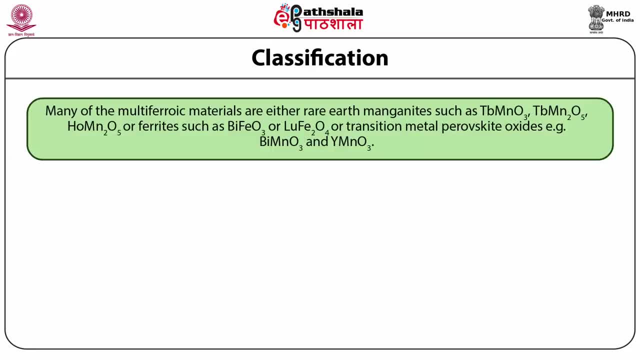 One of them is tetrahy KO3,, which is a magneto-electrolysis which examines the ferrochemical characteristics of metal for sclending. Most of theヨ-n-o-ions that can be obtained from this material are in form of magneto-ectrolysis. 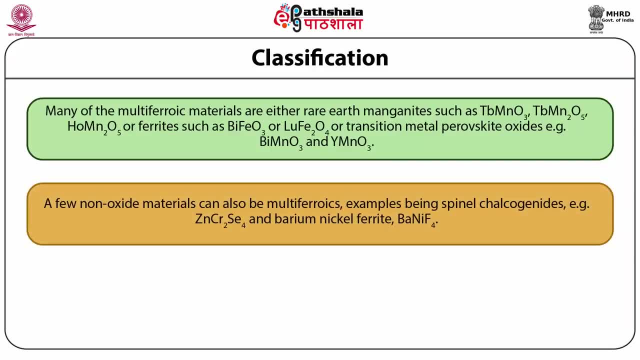 These are non- vagy n-oions. A few non-oxide metal peroskite oxides, For instance b-i-m-n-o-3 and y-m-n-o-3.. materials can also be multi-ferroics, Examples being spinal chalcogenides. 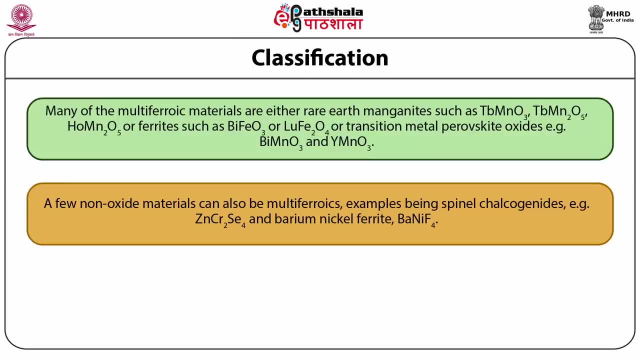 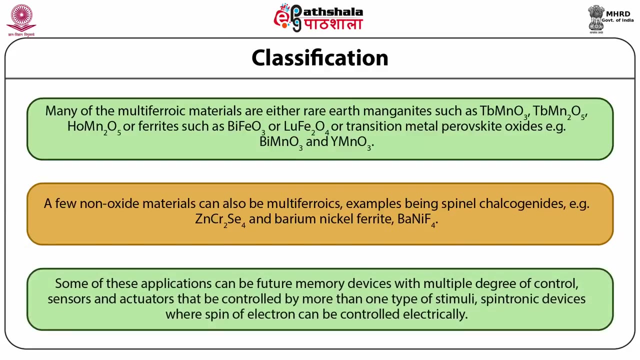 example, zinc, chromium selenide and barium, nickel, ferrite. Given that the multi-ferroic materials show more than one ferroic ordering, the envisaged applications are numerous. Some of these applications can be future memory devices with multiple degree of control. 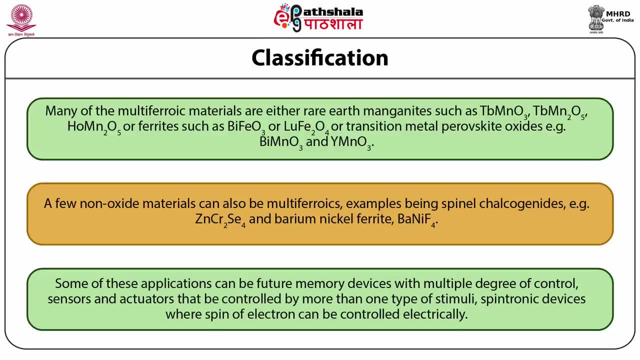 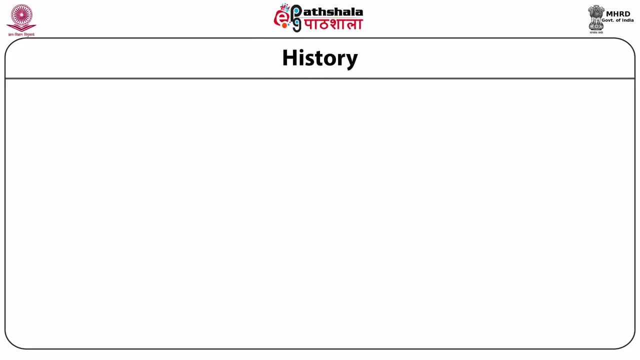 sensors and actuators that be controlled by more than one type of stimuli. spintronic devices, where spin of electron can be controlled electrically. Now, students, let us discuss about the historical perspective of magneto-electric effect. Magneto-electric effect was first observed by Röntgen in 1888 and by Puri Curie in 1894.. 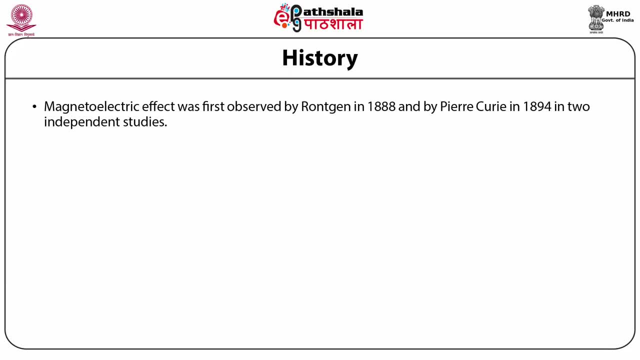 In two independent studies, Röntgen found that a dielectric, when moved in an electric field, became magnetized and conversely, it became polarized when moved in a magnetic field. In contrast, Curie pointed out the relation between the magneto-electric effect. 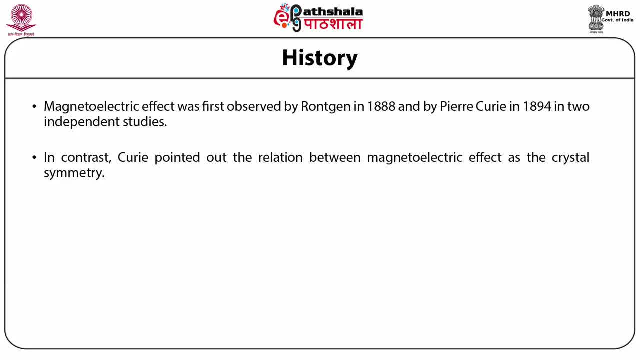 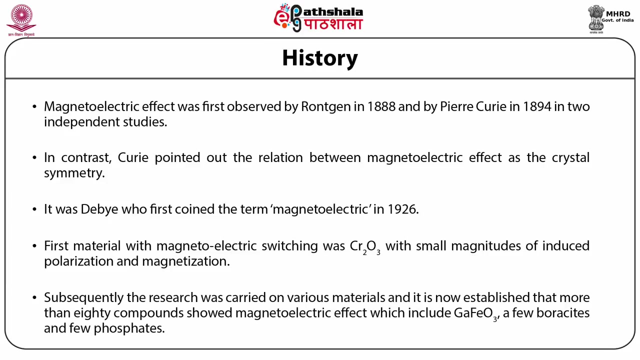 and magnetic field as the crystal symmetry. It was Debye who first coined the term magnetoelectric in 1926.. First material with magnetoelectric switching was chromium oxide with small magnitudes of induced polarization and magnetization. Subsequently, the research was carried on various materials. 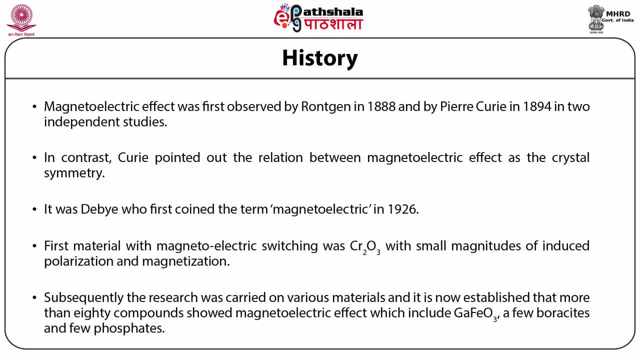 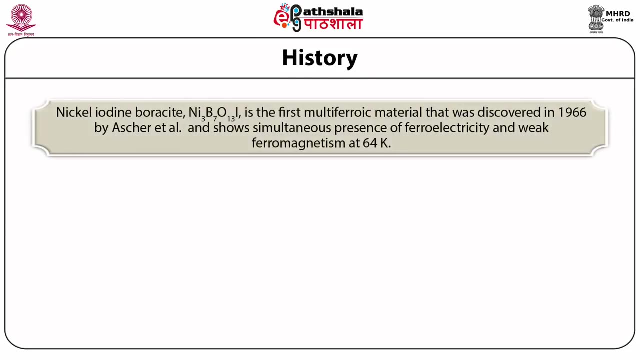 and it is now established that more than 80 compounds showed magnetoelectric effect, which include gallium, ferrite, a few borosaldehyde and a few borosaldehyde, Nickel iodine borosite. Ni3B7O13I is the first multi-ferroic material that was discovered. 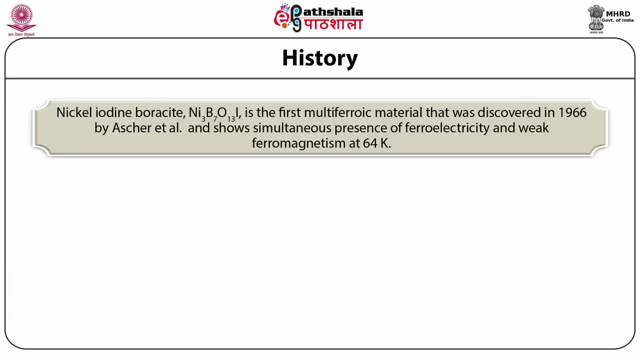 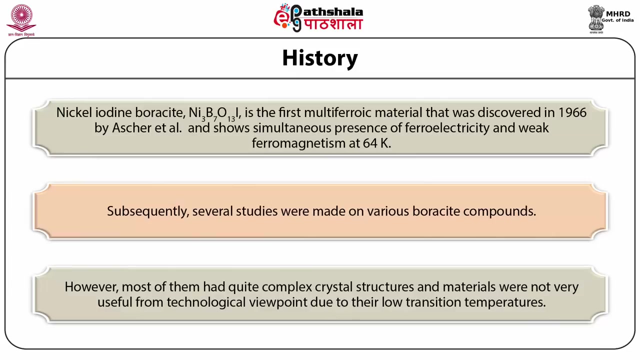 in 1966 by Ascher et al and shows simultaneous presence of ferroelectricity and weak ferromagnetism at 64 Kelvin. Subsequently, several studies were made on various borosite compounds. However, most of them had quite complex crystal structures and materials were. 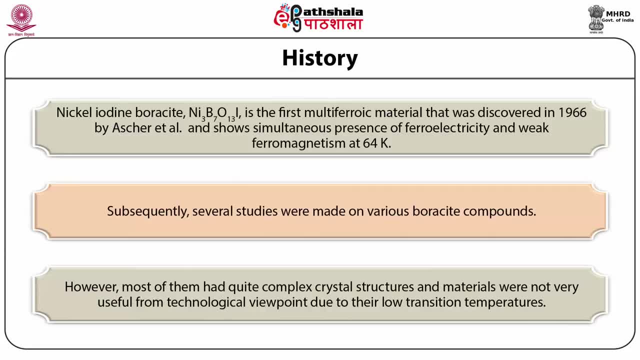 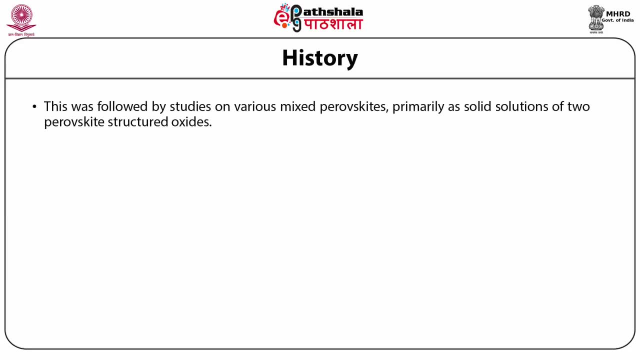 not very useful from technological viewpoint due to the fact that they did not have a very precise low transition temperature. This was followed by studies on various mixed perovskites, primarily as solid solutions of two perovskite-structured oxides. Russian scientists took lead in these investigations, where they replaced some of the deep, counterintuitive possibilities of ferro-gas. 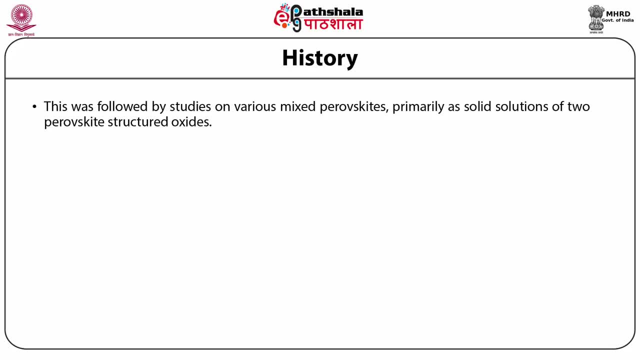 zero type cations in the ferroelectric perovskite oxides with magnetic d n type elements in order to induce magnetic ordering. One of first such compounds was a solid solution of lead based compounds: PbFe2x3, W1x3O3 and PbMg1x2, W1x2O3.. In this solid solution, ferroelectricity is. 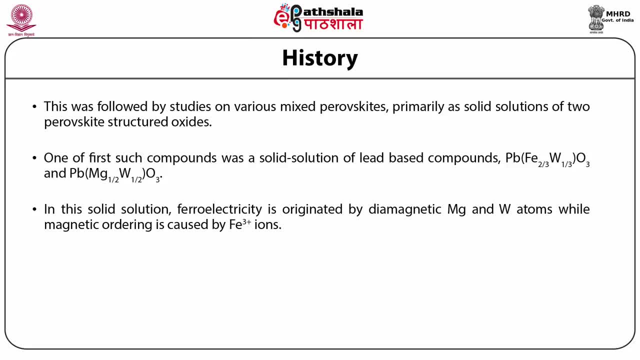 originated by diamagnetic magnesium and tungsten atoms, while magnetic ordering is caused by Fe3 plus ions. A few other candidates which showed ferroelectricity and anti-ferromagnetic ordering were iron or cobalt-doped lead tungstates or lead tantalates. However, most of these materials 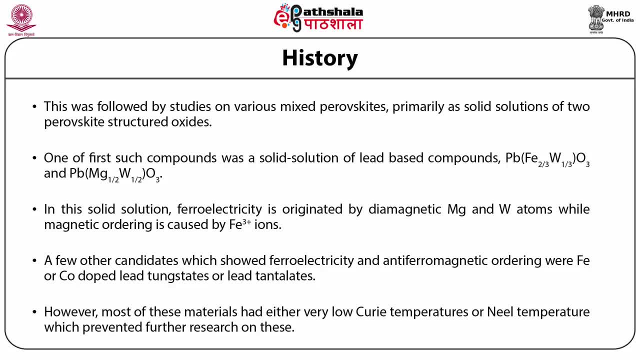 had either very low Curie temperatures or nil temperature in order to induce magnetic ordering. A few other candidates which showed ferroelectricity and anti-ferromagnetic ordering were iron or cobalt-doped lead tungstates or lead tantalates. The latter had either very low Curie temperatures or nil temperature in order to induce magnetic. 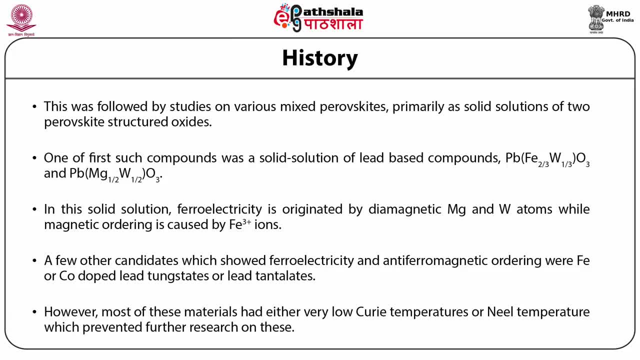 ordering. A few other candidates which showed ferroelectricity and anti-ferromagnetic ordering were iron or cobalt-doped lead tungstates or lead tantalates. A few other candidates which prevented further research on these. Subsequently, the research focus was on other perovskite. 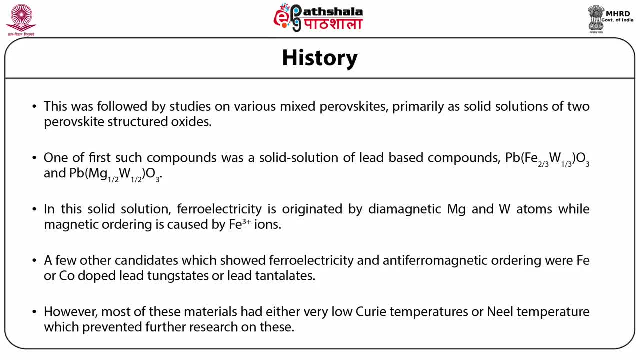 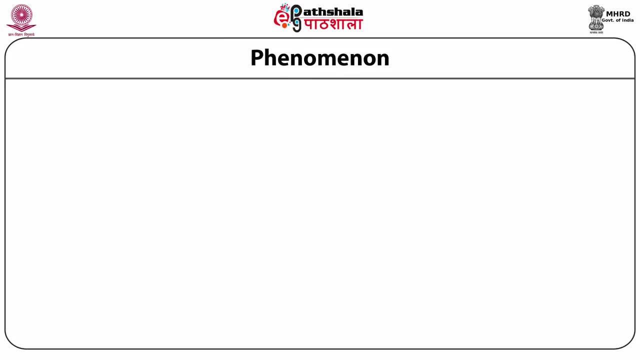 materials which are either manganites or ferrites and have been more promising than previously researched materials, which will be discussed later. Now let us discuss about the requirements for a material to be ferromagnetic, ferroelectric and, finally, the multi-ferroic. 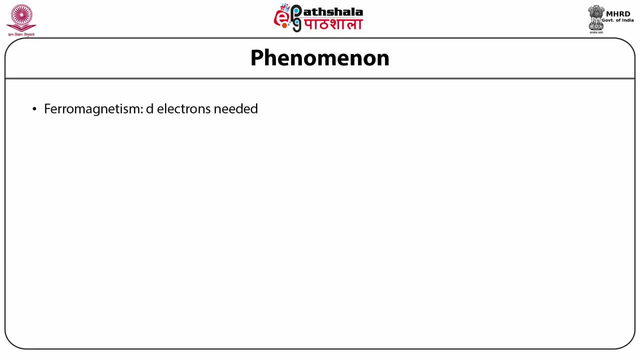 For a ferromagnetic material, the D electrons are needed. That is iron, manganese and nickel and LA and strontium. amino 3 also exhibits the ferromagnetism. For a ferroelectric material, the D electrons are not needed. That is the barium. titanate is the best example. 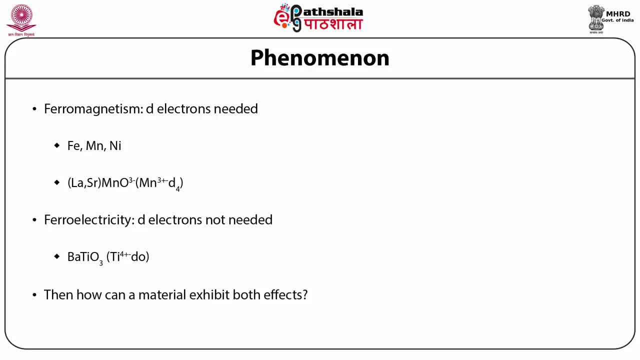 Then the question arises: how can a material exhibits the both the effects. So, students, now we will discuss about the requirements for a material to be multi-ferroic. There are many material requirements which need to be fulfilled for a material to be called as. 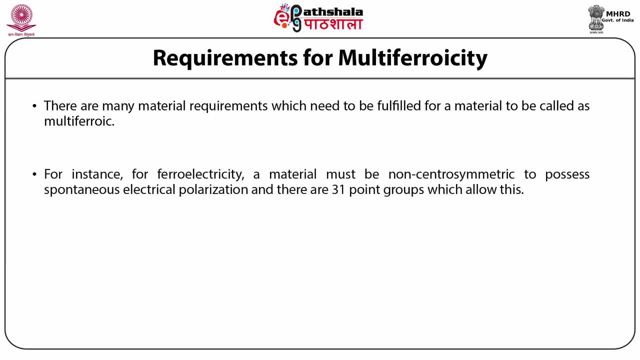 multi-ferroic. For instance, for ferroelectricity, as we have already discussed, it must be non-centrosymmetric to possess the electrical polarization- and there are 31 point groups which allows this- Out of these 13 point groups- allows the occurrence of both the properties simultaneously. 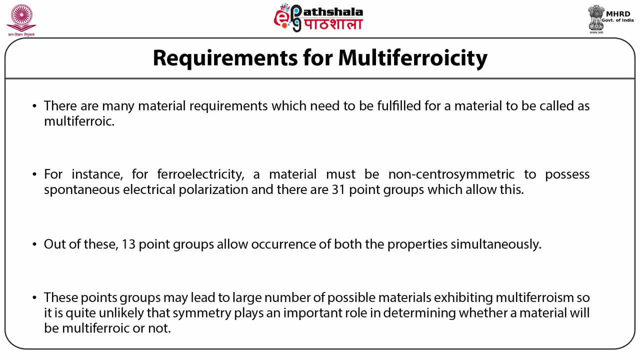 These point groups may lead to the occurrence of both the properties simultaneously. For instance, for ferroelectricity, as we have already discussed, it must be non-centrosymmetric to possess the electrical polarization, and there are 31 point groups which allow this. 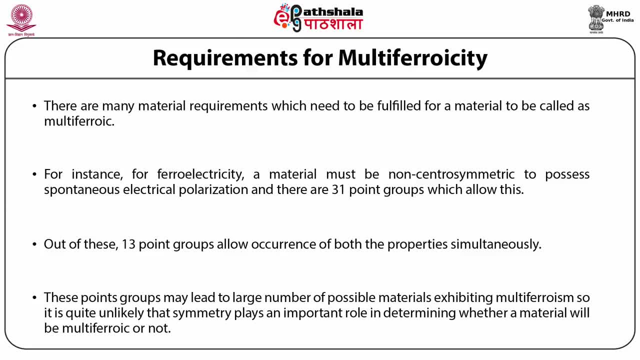 Out of these 13 point groups may lead to the occurrence of both the properties simultaneously. Large number of possible materials exhibiting multi-ferroism. so it is quite unlikely that symmetry plays an important role in determining whether a material will be multi-ferroic or not. 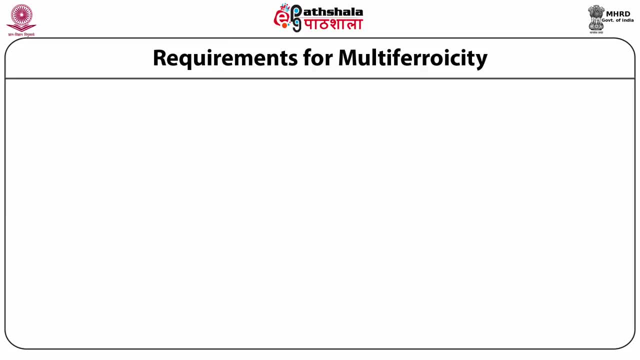 There are contradictions in terms of the requirement of functionality. Electrically speaking, one requires a ferroelectric material to be the insulator, while it is not a constraint for a ferromagnetic material. For the most ferromagnets, high electrical conductivity is due to higher number of free 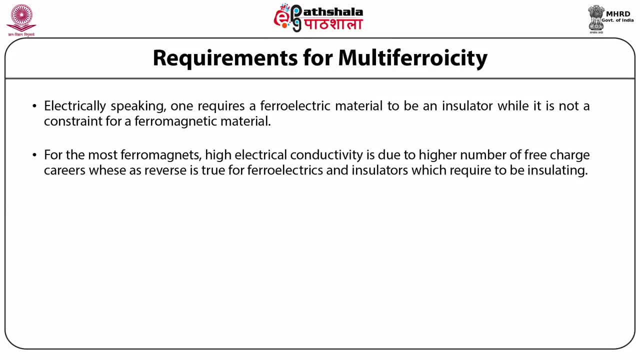 charge carriers, whereas reverse is true for ferroelectrics and insulators, which require to be insulated. However, a few magnetic oxides, eg half-metallic magnets and ferrimagnetic oxides, exhibit reasonable spontaneous magnetism whilst simultaneously being semi-conducting or insulating. 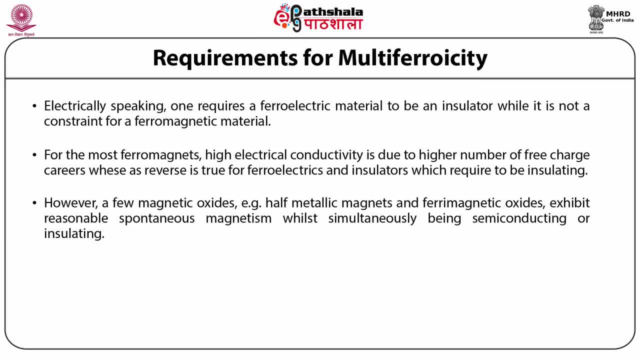 As far as chemistry of the material is concerned, most우 ferroelectrics require ions whose shells are filled. If the material has perovskite structure, then the B atom at the center of BO6 octahedra must have filled D shells, ie has D0 type. 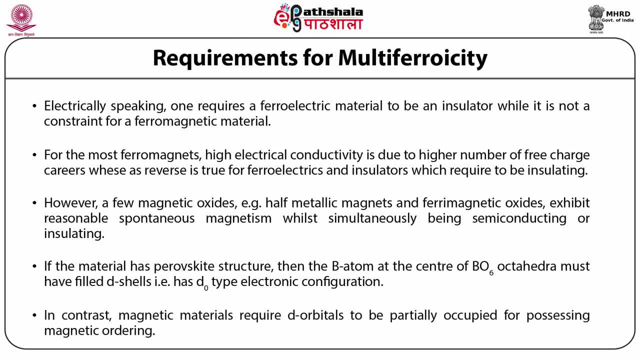 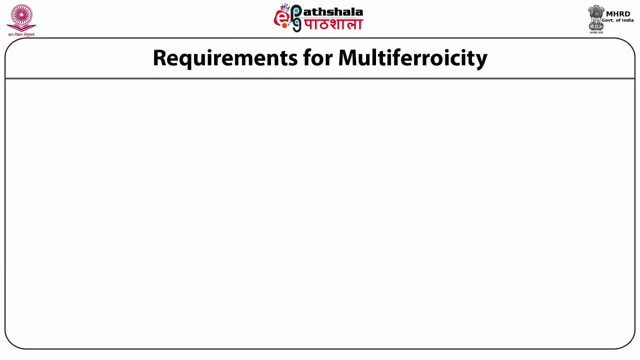 EVs. In contrast, magnetic materials require D orbitals to be partially occupied for possessing magnetic ordering. Latter also imposes constraints to maintaining the centre of symmetry in these systems. Another factor that could be analyzed in battery-powered electronic 9V power station is the size of 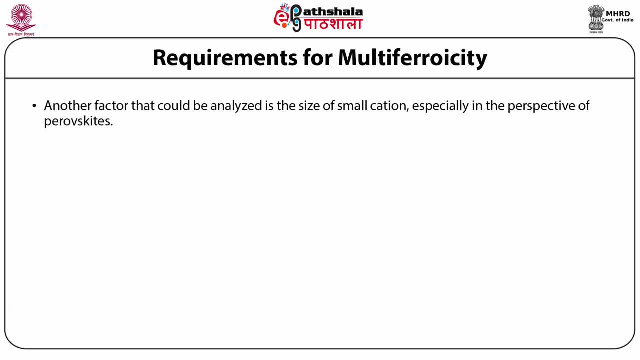 small components, cation, especially in the perspective of perovskites. However, upon comparison one finds that this is not a valid argument, as sizes vary considerably for kinds of compounds. Another contrast between ferroelectric and ferromagnetically ordered system: 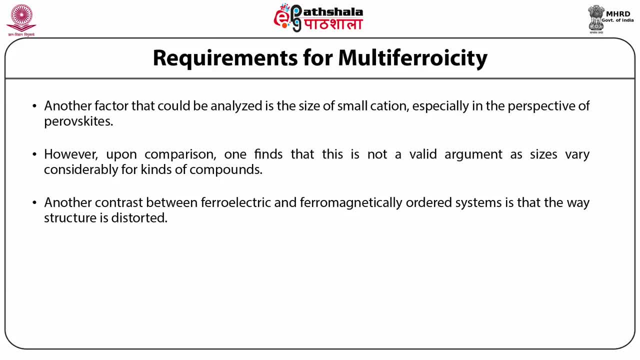 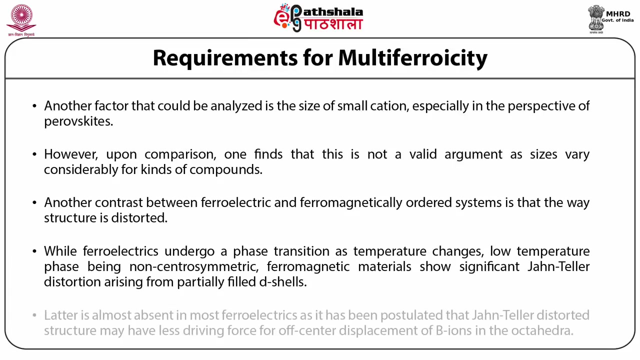 is that the wave structure is distorted while ferroelectrics undergo a phase transition as the temperature changes. Low-temperature phase being non-centrosymmetric, ferromagnetic materials show significant John-Taylor distortion arising from partially filled veins. The latter is almost absent in most ferroelectrics, as it has been postulated that John-Taylor 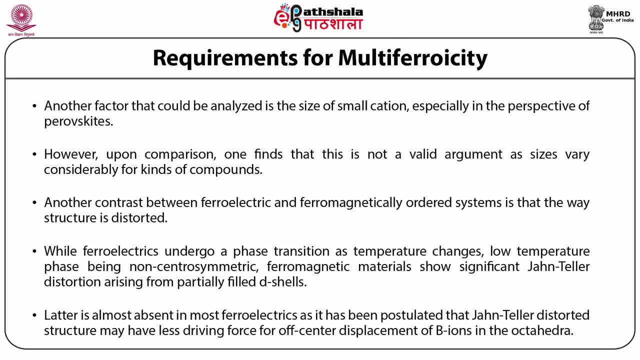 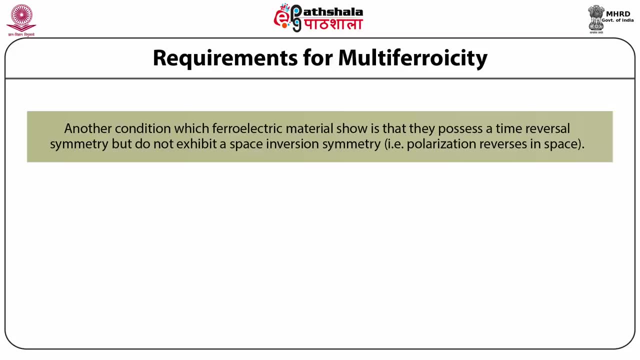 distorted structure may have less driving force for off-center displacement of B ions in the octahedra. Another condition which ferroelectric materials show is that the whole structure is not fully constructed, and in fact the entire structure is not fully constructed In the case of ferroelectrics. ferro-magnetic materials possess a time-reversal symmetry. 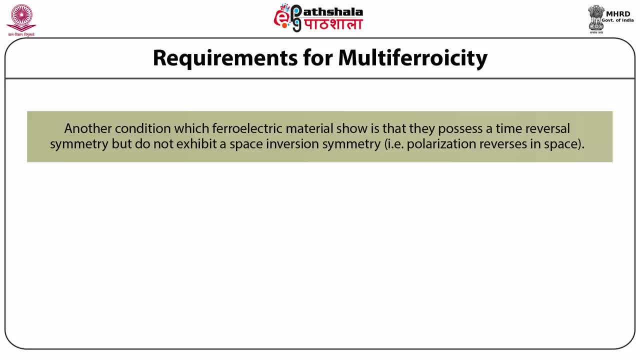 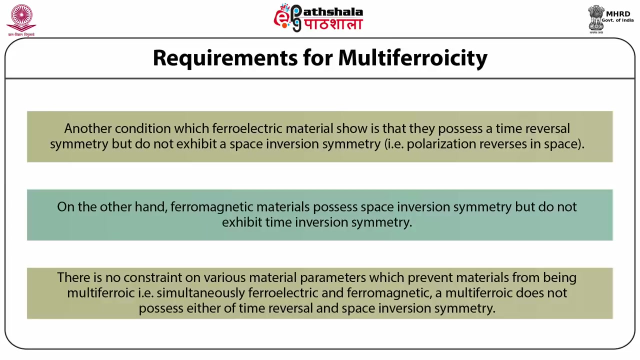 but do not exhibit a space-inversion symmetry. On the other hand, ferro-magnetic materials possess the space-inversion symmetry but do not exhibit the time-inversion symmetry. So now to conclude that there is no constraint on various material parameters which prevent 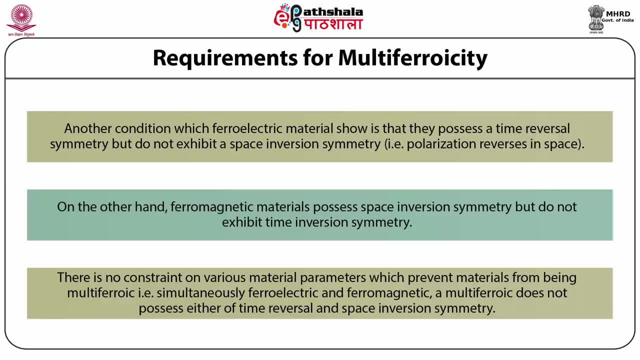 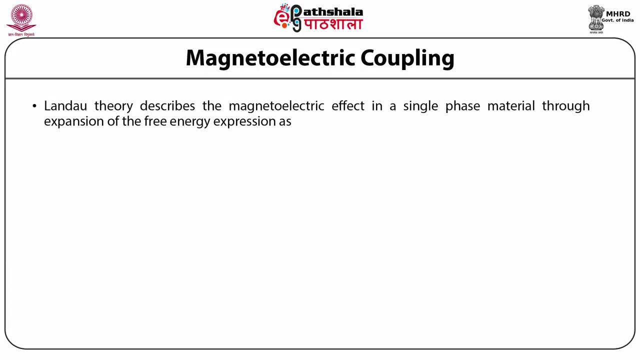 the materials from being aesthetic and time-inversion. from being multi-ferroic, ie simultaneously ferroelectric and ferromagnetic. a multi-ferroic does not possess either of time reversal and space inversion symmetry. Magneto-electric coupling: According to Landau theory, the magneto-electric 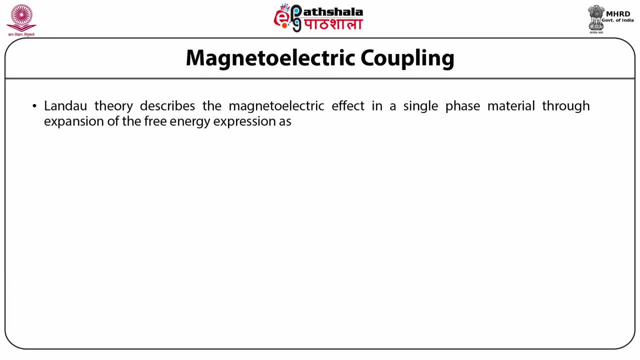 effect in a single phase. material can be described through the expansion of the free energy as F as a function of E and H is equal to F0 minus Pi S multiplied by Ei minus Mi S multiplied by H2.. EIHJ minus half of epsilon-naught, epsilon-IJ, EIEJ minus half mu-naught, mu-IJ, HIHJ minus. 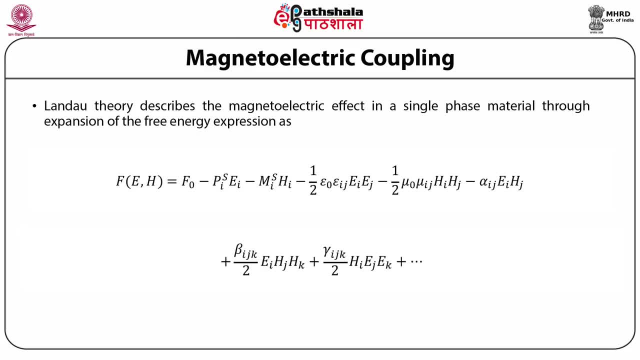 alpha-IJ EIHJ plus beta-IJK by 2, multiplied by EIHJ EIHJ minus half of epsilon-naught, epsilon-IJ EIHK plus beta-IJ EIHK by 2 plus so on. where EI is the ith component of E and HI is the ith component of H, are the electric. 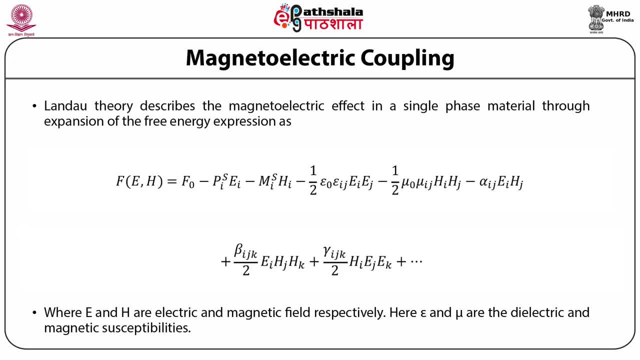 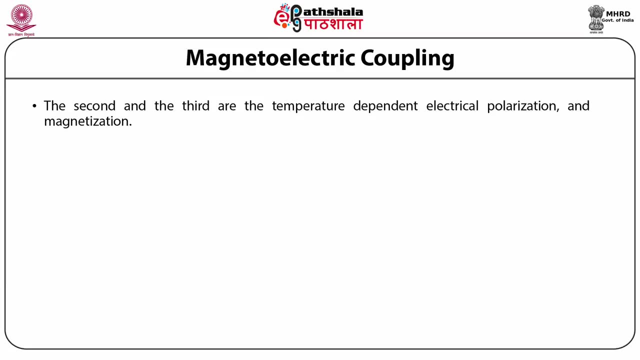 and magnetic fields, while epsilon and mu are the dielectric and magnetic susceptibilities respectively. The second and the third term in these equation denotes the temperature dependent electrical polarization, corresponding to EI and PIS, and magnetization corresponds to HI and MIS, respectively. Fourth and the fifth. 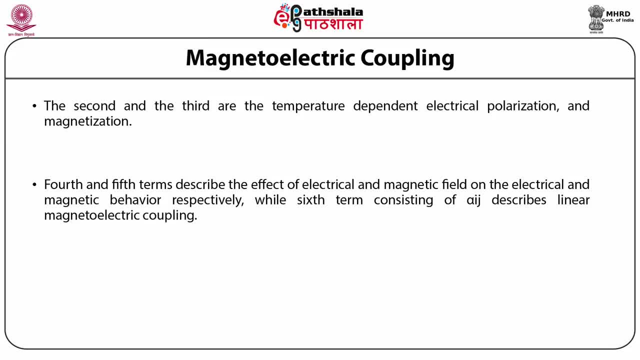 terms describes the effect of electrical and magnetic field on materials, electrical and magnetic behavior respectively. Here epsilon iJ and mu iJ are second-rank tensile quantities and is usually independent of EI or HI in the material in STD without the corresponding ferroic ordering. The sixth term consisting of 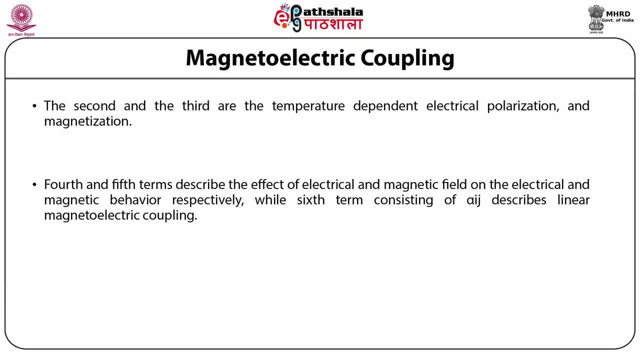 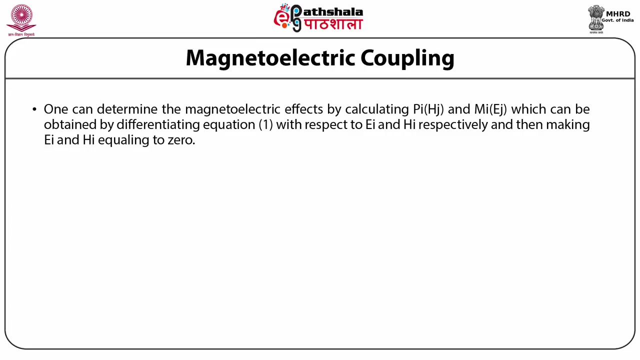 alpha ij describes the linear magneto-electric coupling and is typically of interest, and the next two terms, which consist of beta ijk and gamma ijk, are the third rank tensors and represents higher order magneto-electric coupling coefficients. now one can determine the magneto-electric effects by calculating pi as a function of HJ and MI as a. 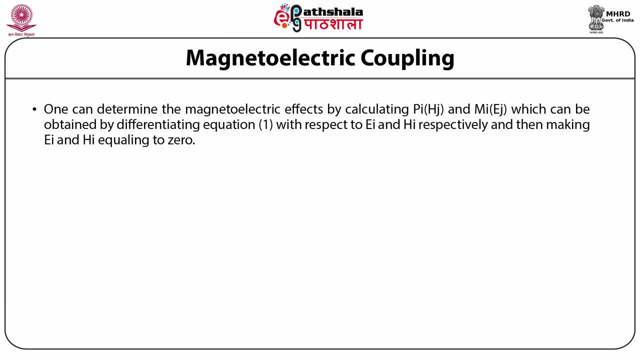 function of EJ, which can be obtained by differentiating the previous information from the previous information, The third term consisting of equation with respect to ei and hi respectively, and then making ei and hi equating to zero, This yields: pi is equal to minus del f by del i, which is equal to pi s plus epsilon. 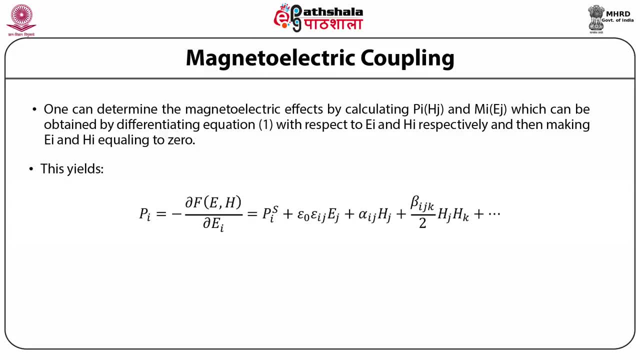 naught epsilon ij ej plus alpha ij hj plus beta ijk by 2 hj hk plus so on. and mi is equal to minus del f by del hi, which is equal to mi s plus mu. naught mu ij hj plus alpha ij ei plus beta ijk ei hj plus so on. 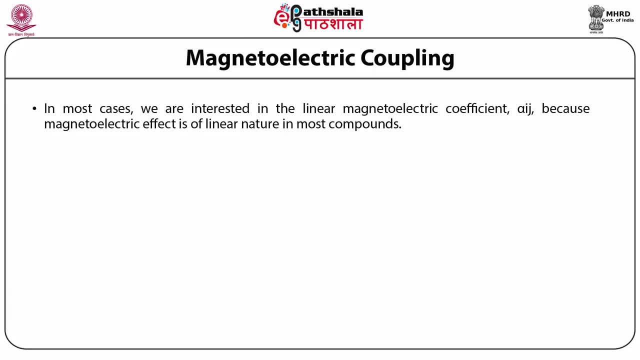 In most cases we are interested in the linear magneto-electric coefficient ie, alpha ij, because magneto-electric effect is of linear nature in most compounds. This coefficient allows one to quantically calculate the magnetic force of the magneto-electric effect. 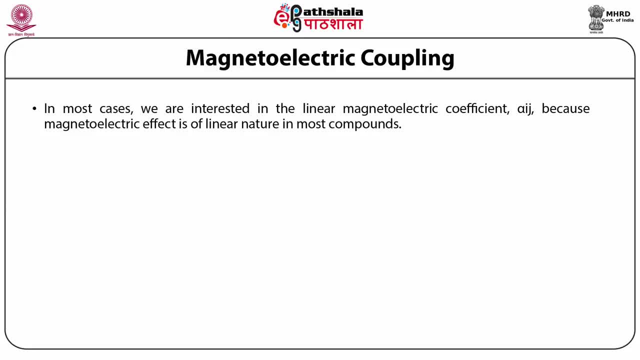 This coefficient allows one to quantically calculate the magnetic force of the magnetic field. In the case of multi-ferroics having both ferroelectric and ferromagnetic ordering, large linear magneto-electric effects are usually expected, because such materials often 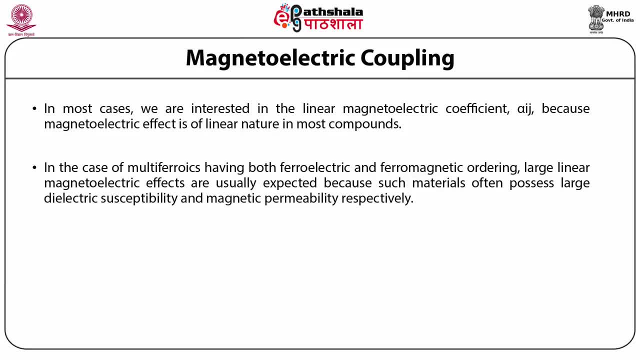 possess large dielectric susceptibility, susceptibility and magnetic permeability respectively. The limit of linear magnetoelectric coefficient is expressed as alpha square ij is less than or equal to epsilon naught mu naught. epsilon ij mu ij. So, students, let us summarize what we have learned in this. 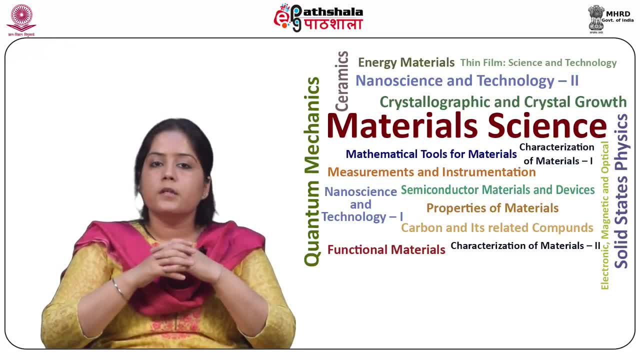 module. First: the multipheroic materials, which are modern materials where one absorbs the coupling of functional order parameter in a single phase. Second: magnetoelectric materials are those materials that are simultaneously electrically and electrically and magnetically polarizable and are not necessarily multipheroic. Third: magnetoelectric